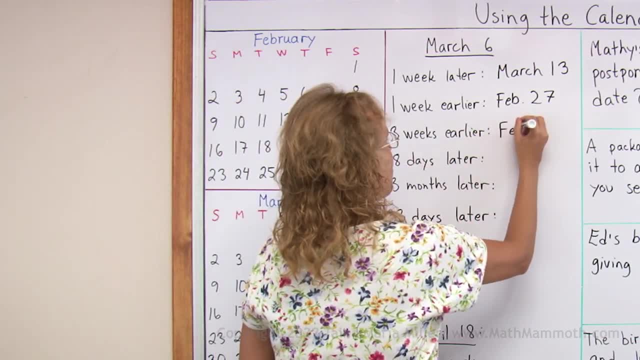 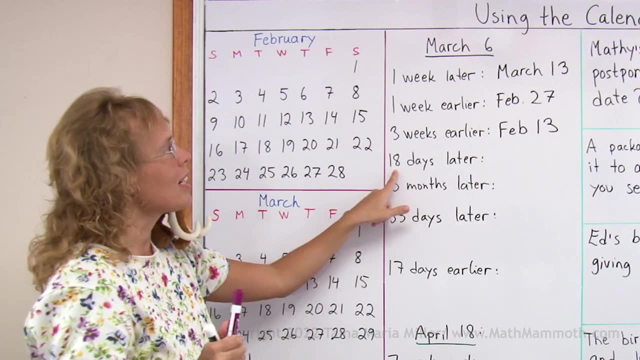 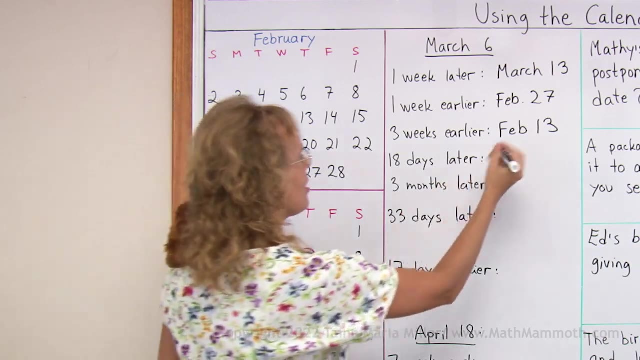 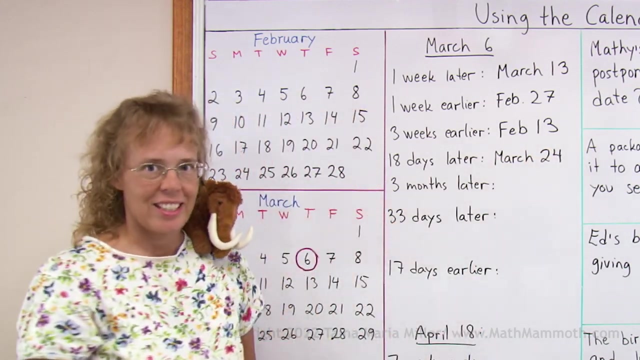 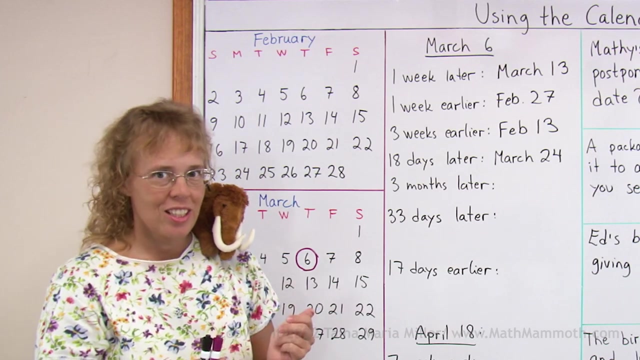 So February 13.. 18 days later: Okay, Let me see if I can just add the 6 and the 18.. Yep, That's 24.. That works fine. So it is March 24.. Three months later: Okay, This time you can count the months. Okay, We are in March and 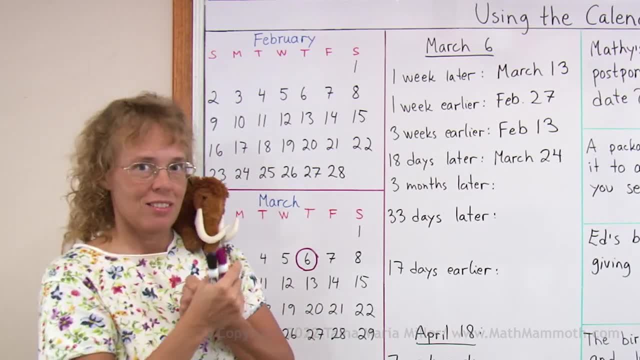 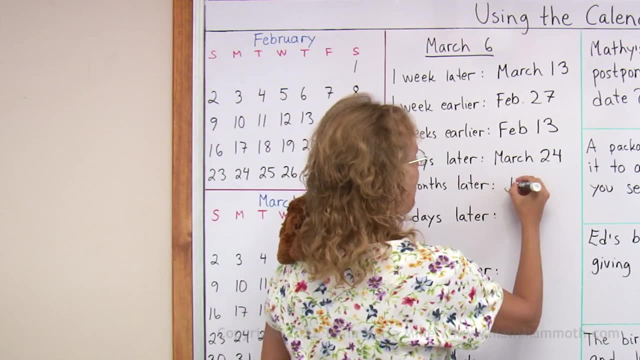 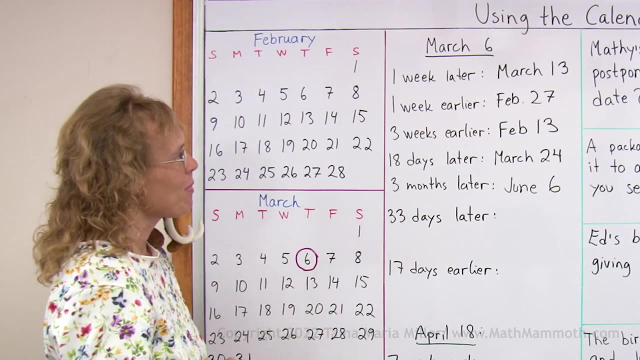 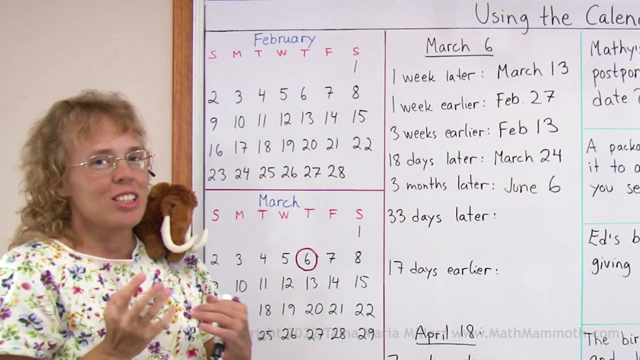 then count three months forward, You would have April, May and June. So three months later is June 6th, 33 days later than March 6th. Okay, Now my addition doesn't really work, because if I add 33 and 6, I get 39., But there is no such date as March 39th. 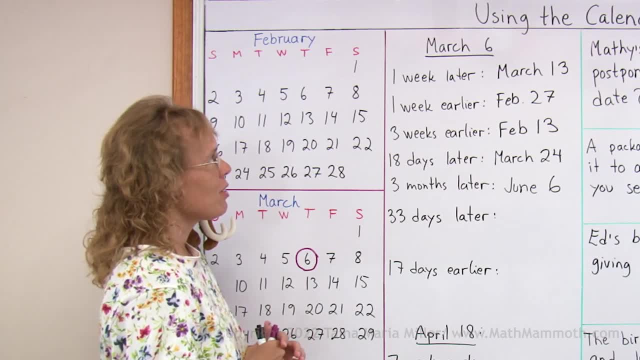 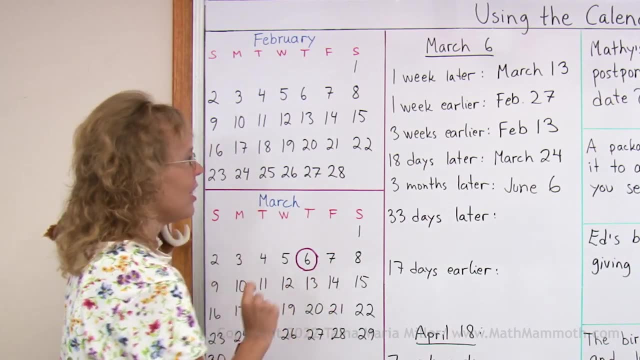 So this is what I would do. I would go on the calendar thirty three days later. But to my But, to make it quicker, I don't have to count like one, two, three, four, five, dah dah, I can go by sevens, because here's seven days later, right? 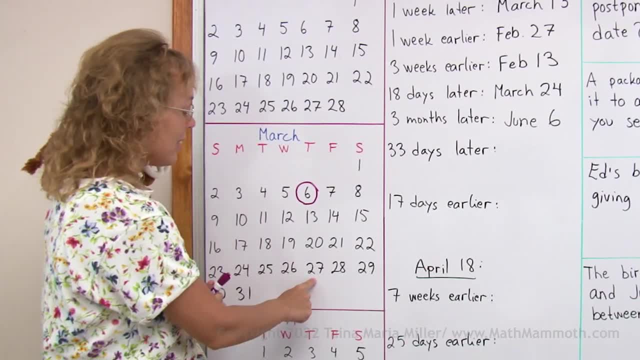 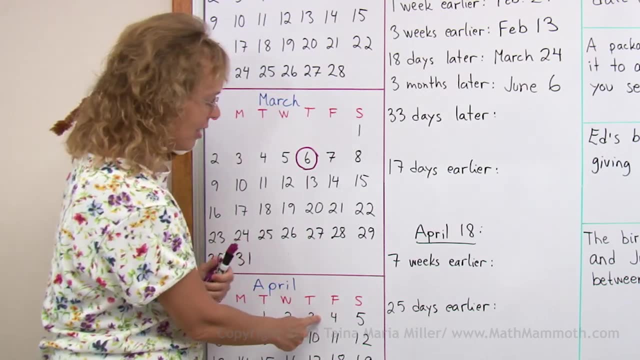 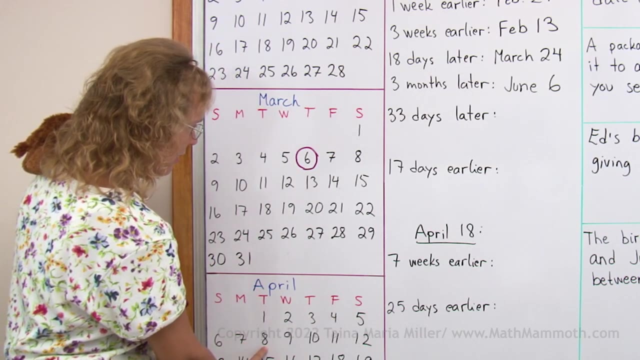 And then this would be 14 days later, 21 days later, and then over here 28 days later. Now we're really close to 33.. So this is 28 days later: 29,, 30,, 31,, 2, and 3.. 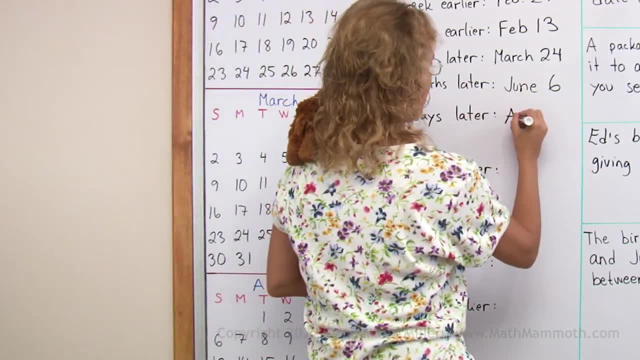 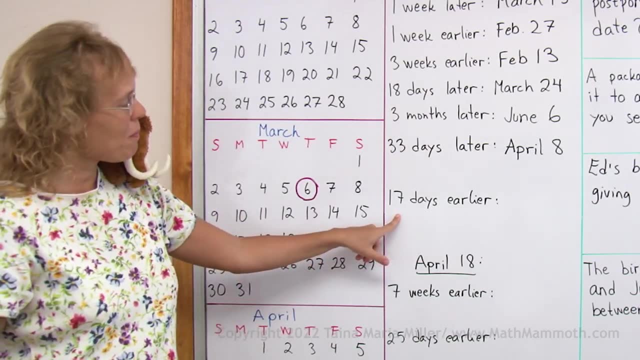 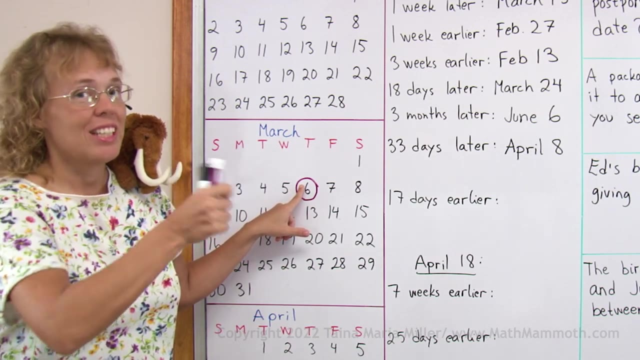 So April 8th, 17 days earlier than March 6th, Okay, we're here. I can count backwards 17 days, but it's quicker to count by sevens, by whole weeks. So seven days earlier is exactly here, right. 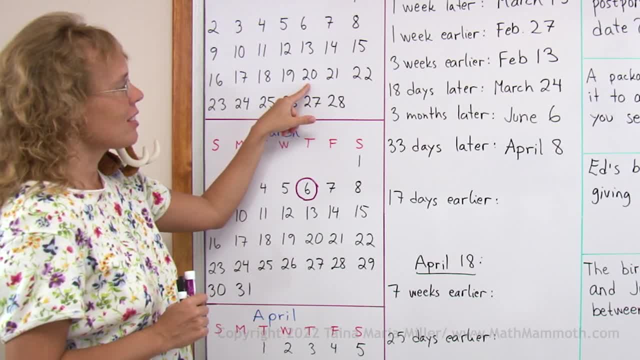 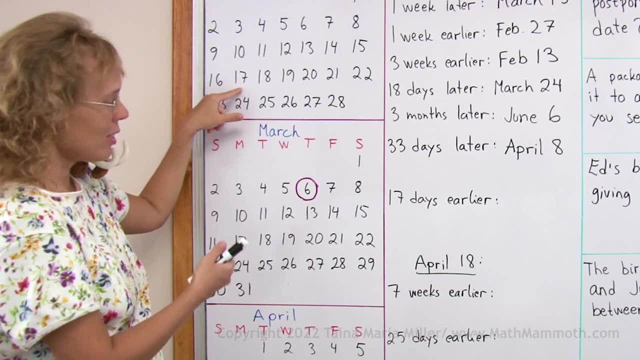 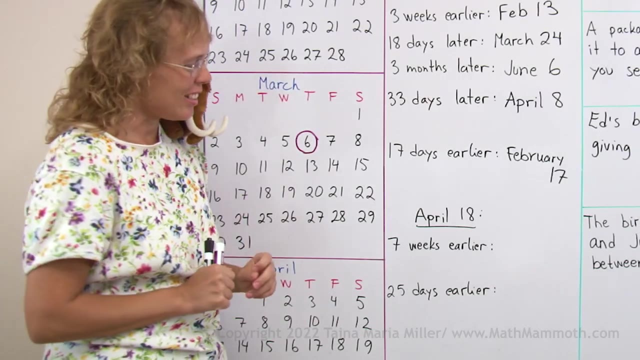 And then another seven days or 14 days earlier is this, And then I go backwards three more days. That's 15,, 16,, 17.. So that is February 17th. All right, maybe you can try this now. 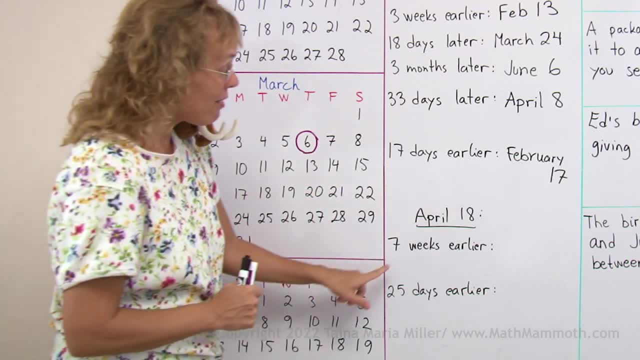 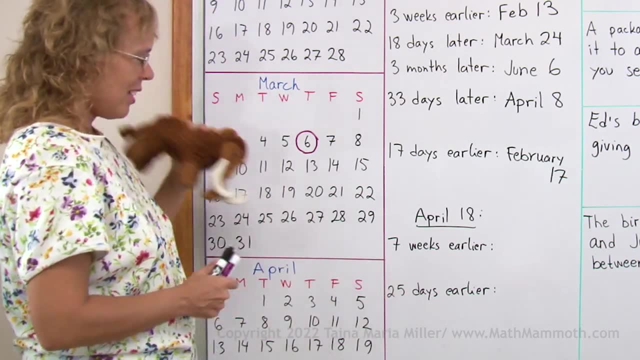 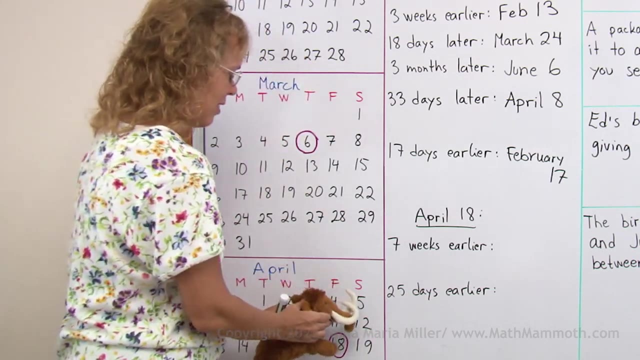 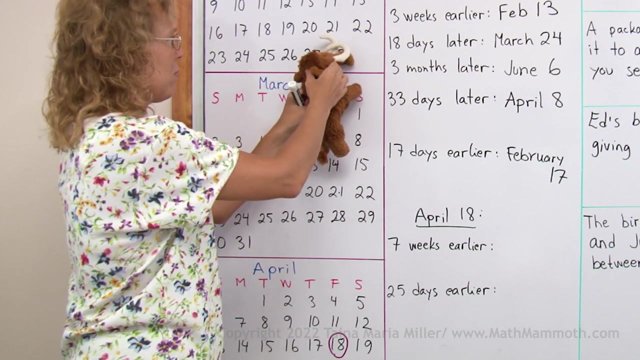 April 18th, And then what date would we have seven weeks earlier? What would you do, Matthew? you want to show them April 18th? aha, Matthew finds it. And then Yep, go seven weeks earlier. What do you think? 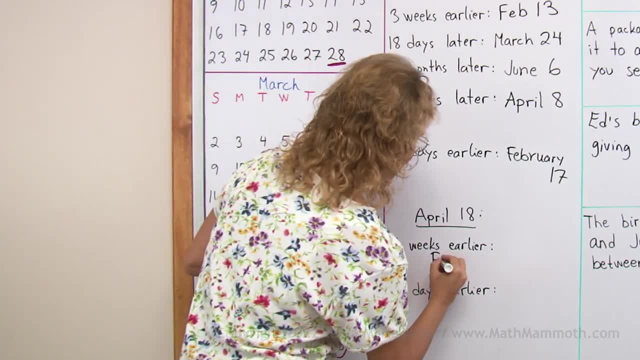 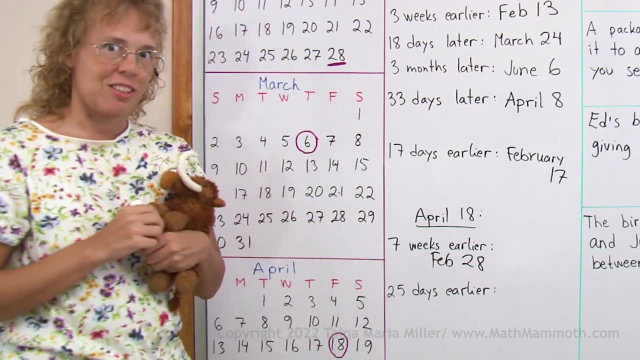 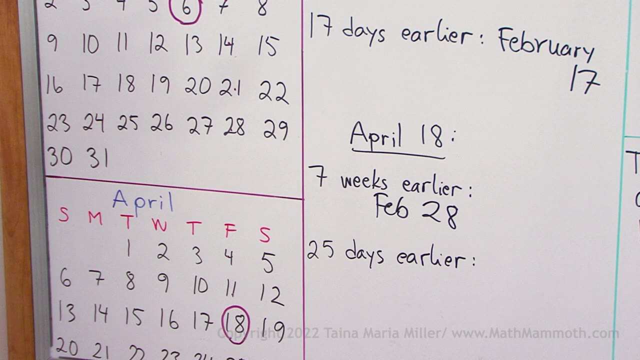 Did Matthew do it right? February 28th Looks like it Friday. Friday, 25 days earlier. How would you find that out? If we are here at April 18 and you need to find a date that is 25 days earlier, what? 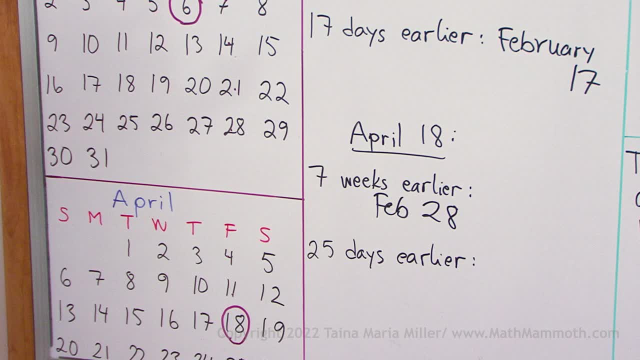 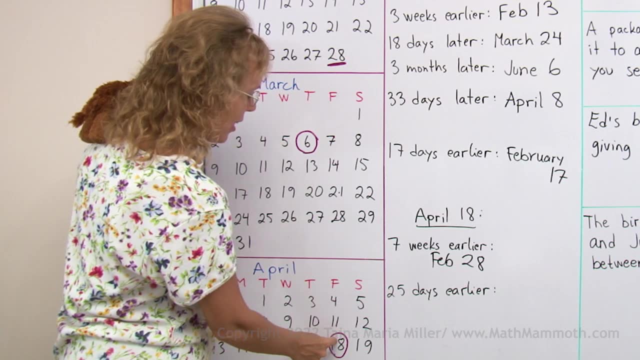 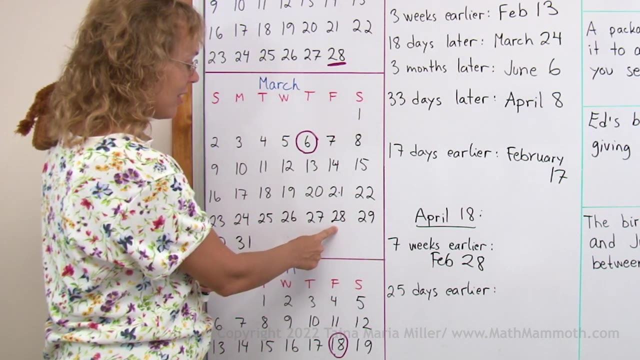 shall you do? My method was that I count by sevens, by weeks. So here's seven days earlier, and here's 14 days earlier, and here's 21 days earlier, and then 22,, 3,, 4, and 5.. 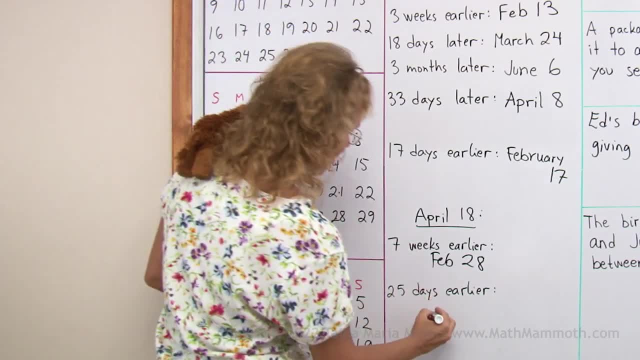 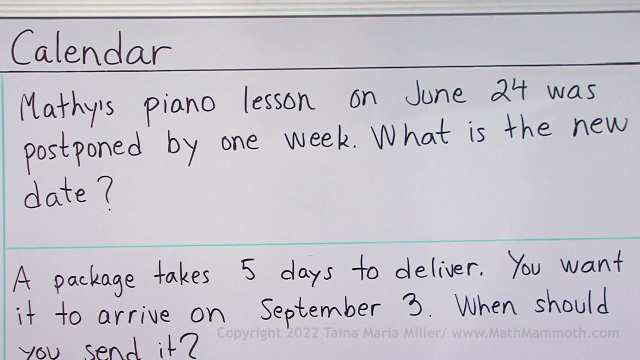 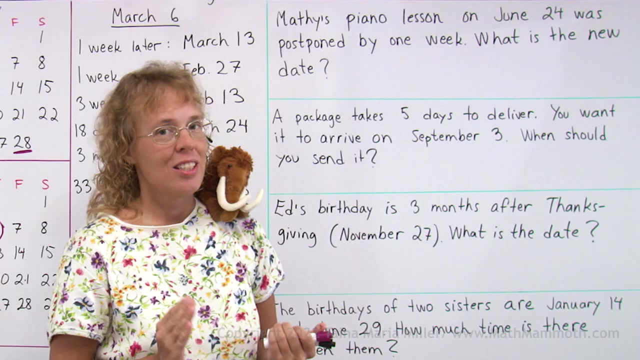 This one here, March 24th. Matthew's piano lesson on June 24th was postponed by one week. What is the new date? Okay, One week is seven days, So all we really need to do, looks like, is just add 7 and 24.. 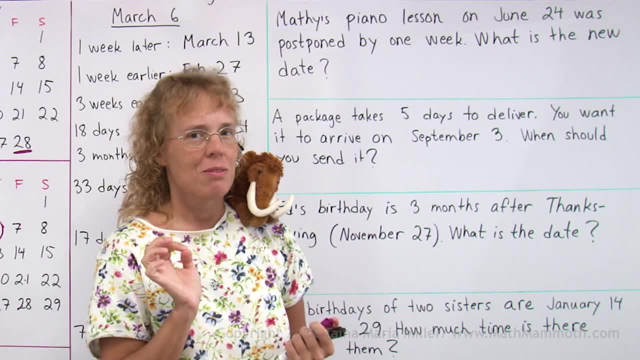 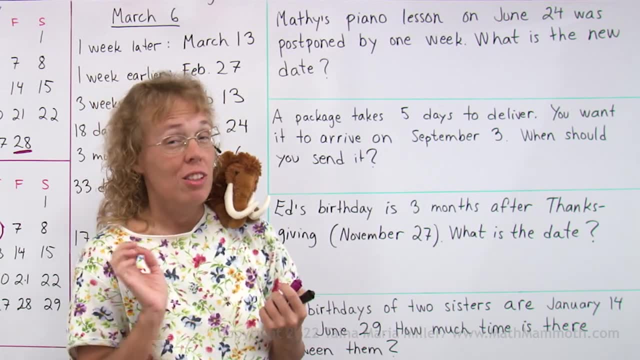 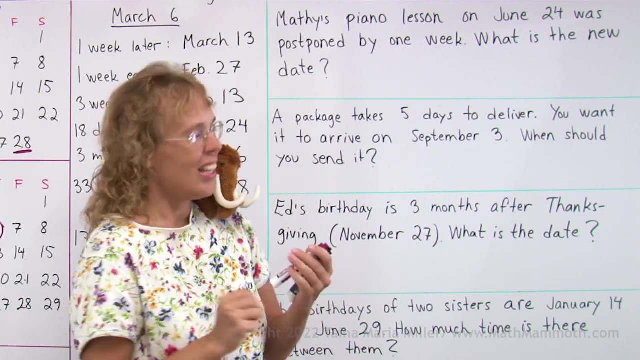 So we would get June 31,, June 31st. But there's one problem here. Do you know that? It is that June does not have 31 days. June only has 30 days. okay, So there is no such date as June 31st. 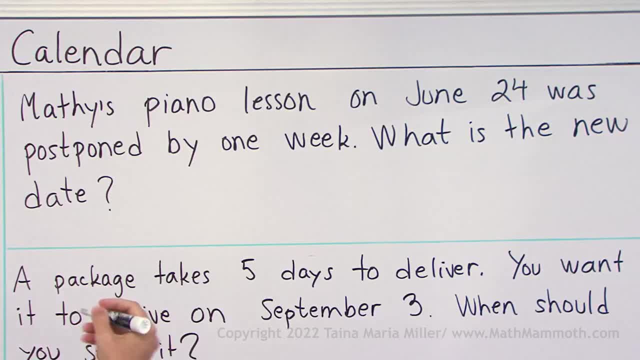 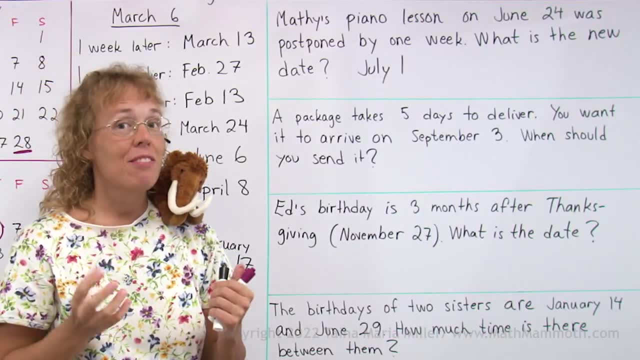 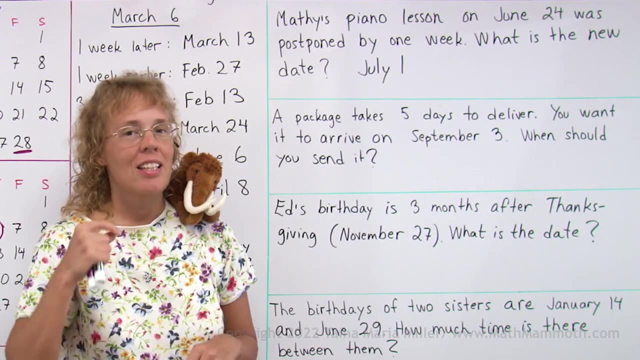 It is instead the first day of July. You need to remember what months have 31 and what months have 30 days. okay, The ones having 31 days start with January and then they are every other month, except it switches with July and August. So that July and August both have 31, and then after that it again is every other month having 31 days. Okay, A package takes five days And you want it to arrive on September 3rd. When should you send it? 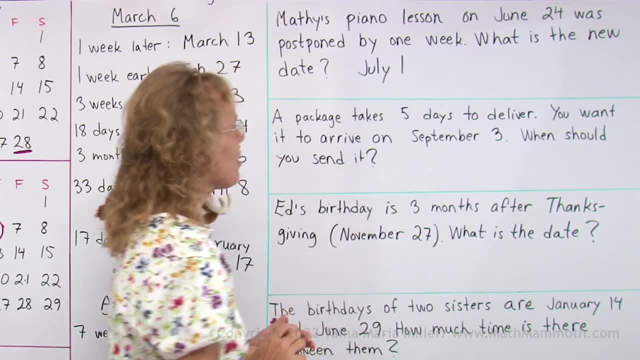 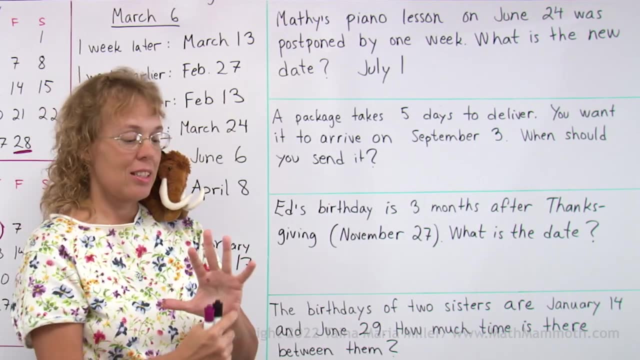 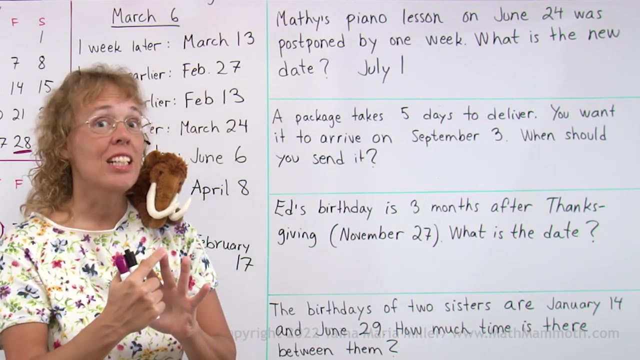 Okay, Five days earlier than September 3rd. Let's use our five fingers and count backwards, right? Okay, We would have September 2nd, September 1st and then August. what? What's the last day of August?